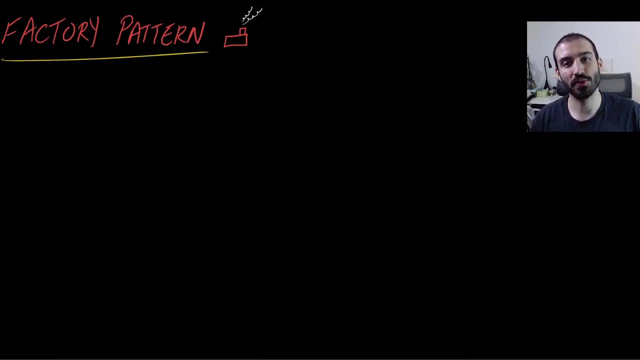 What is going on? everyone? In this video we're going to be talking about the factory pattern in the context of this book, which is Head First Design Patterns, And this video is part four of a video series that I'm doing on every design pattern from this book. So previously I've done 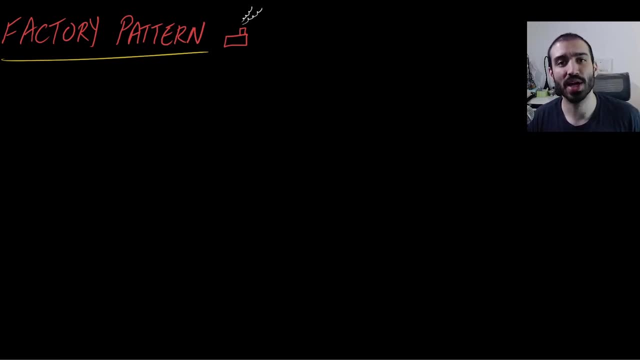 the observer pattern, the decorator pattern and another one as well. But if you're interested in watching those videos, I'll put them down below. But today we're going to be talking about the factory pattern, And I'm particularly excited about this video because I personally feel that 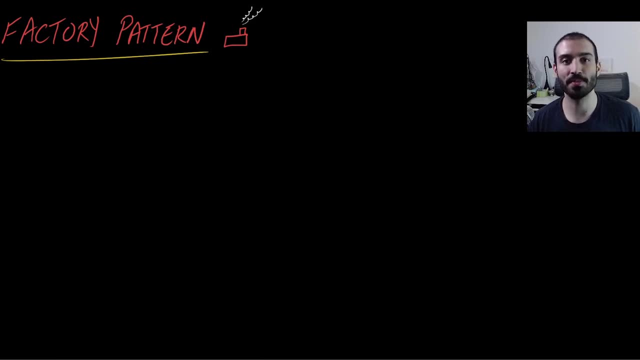 the factory pattern is one of the most useful design patterns in all of software design, And I say that because it's one that I tend to use the most frequently. It simplifies your code in a lot of different ways, and we're going to see some examples of that in a few moments here. 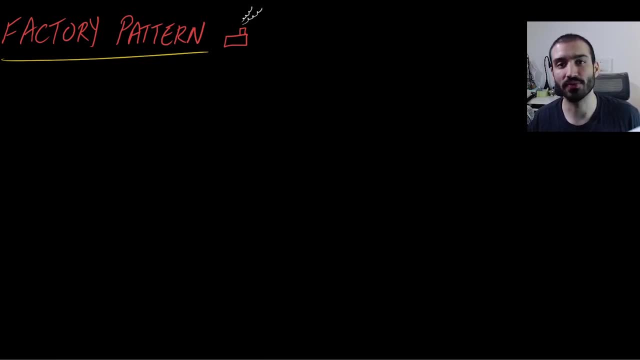 So, in terms of the agenda of this video, first I'm just going to define what the factory pattern is, as per the definition of this book, Just talk about it a little bit and just make sure that you're familiar with what it is. So let's get started. 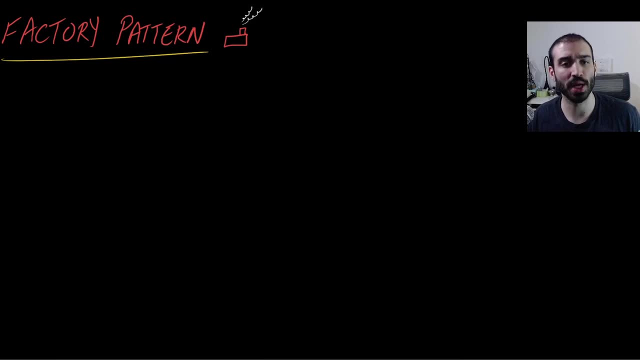 Make sure that you grasp the concept and just do a quick little prototype example just to show you exactly what I mean. From there we're going to go into some more sophisticated class diagrams using a different example, And then I'm going to show you how you actually implement it using Java as 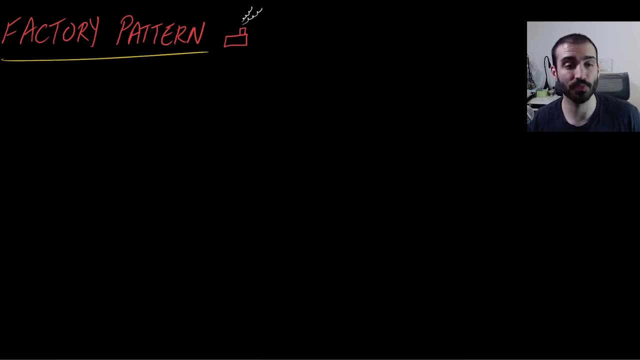 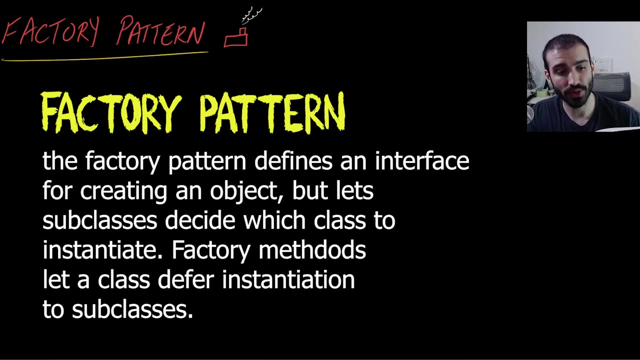 a programming language And for that part I'm going to bring you over to my IDE. So, as per the definition in this book, the factory pattern defines an interface for creating an object, But let subclasses decide which class to instantiate Factory methods. let a class defer instantiation to subclasses. 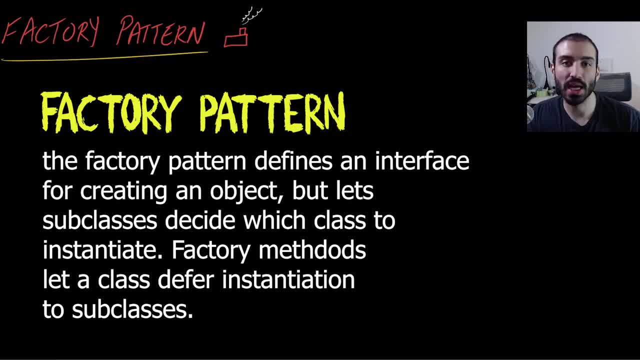 So let's tease this definition apart a little bit. In the beginning we're saying that we'd want to define an interface for object creation. So right off the bat we know that we're going to be creating an object that contains logic on how to create other objects. So that's the first part of 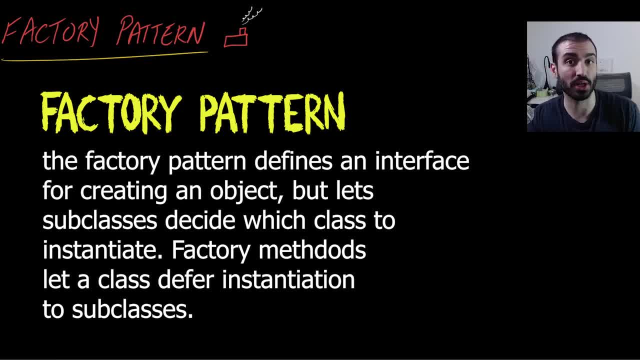 the factory pattern. It's essentially a object that knows how to create other objects. So that's the first part of the factory pattern. It's essentially a object that knows how to create other objects. So that's the first part of the factory pattern. It's essentially a object that knows how to. 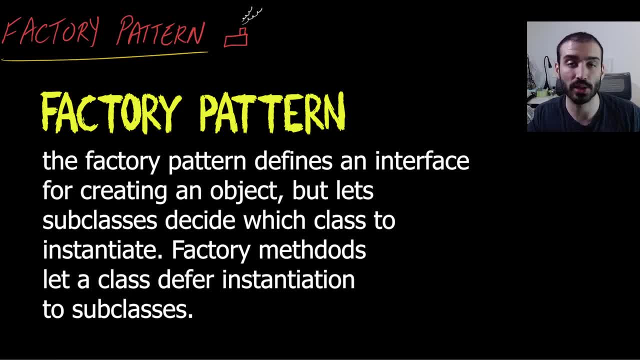 construct other ones And it has specific logic that's built in it so that it can do it pretty intelligently. And the second part says that the factory method lets a class defer instantiation to subclasses, And what this is essentially saying is that you can let subclasses decide. 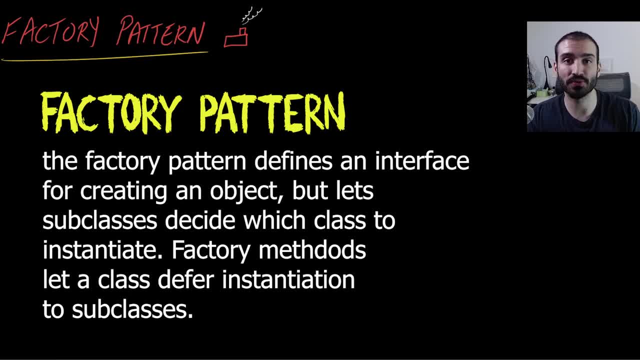 which type of object that you want to create. The factory can just define the interface that you want the subclasses to follow, but it doesn't necessarily know how the subclasses implement or the core logic that exists within those subclasses. So this was a pretty crude. 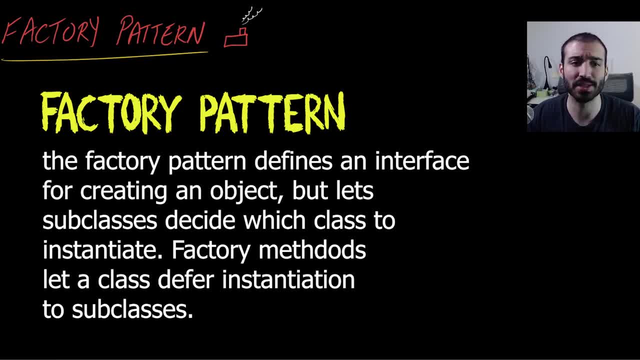 definition of the factory method. But let's tease this definition apart a little bit. In the beginning definition: I don't expect you to understand the factory pattern just based off that. So now what I want to do is just go through a pretty trivial example. 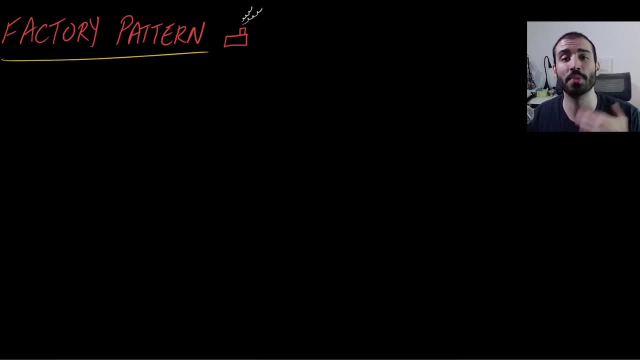 of what I call the simple factory pattern, or the most basic factory pattern that you can define while still being able to call this a factory pattern. So let's assume that we're working with an example where we're working in the domain of credit card transactions. 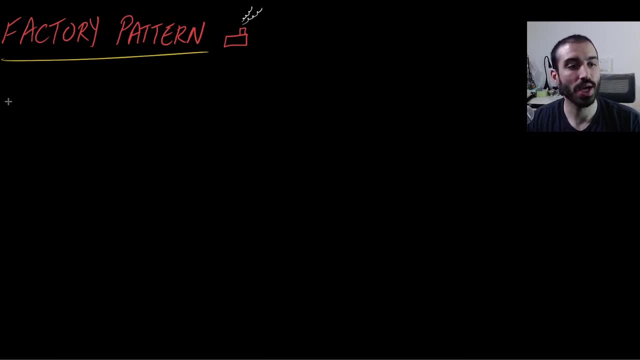 So let's say, in this problem you have two types of transactions. The first one is a purchase transaction And the second is a refund transaction. You're buying stuff or you're refunding stuff. Now let's say that you are building an API And your API is going to take. 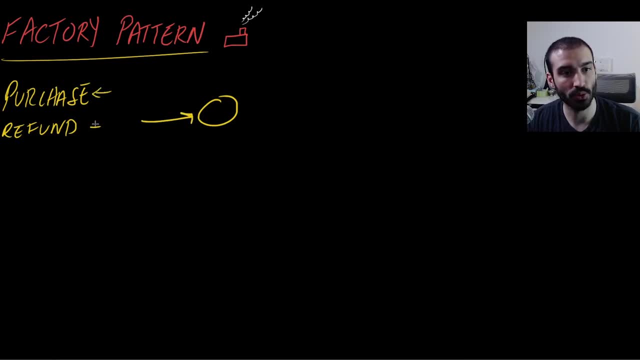 in one of these two different types, either a purchase or a refund. Maybe this API is called process transaction, So let's name this thing process transaction And let me just grab a different color here to indicate the payload. So let's say the contract. 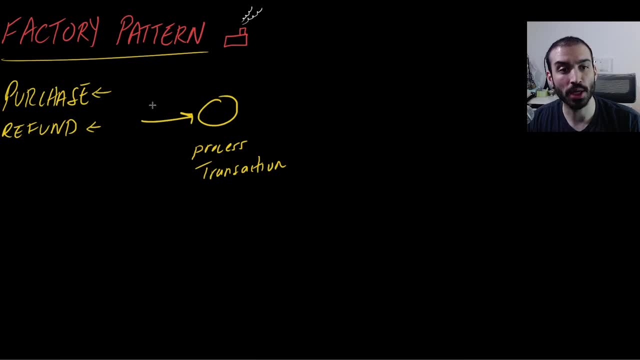 of this API. by the way, this is an API, if that's not already clear. it takes an input argument called type, And type can be a string, And that can be either a purchase or a refund. So this is all well and good. We have this API here that takes in a type and it's focused on the purchase. 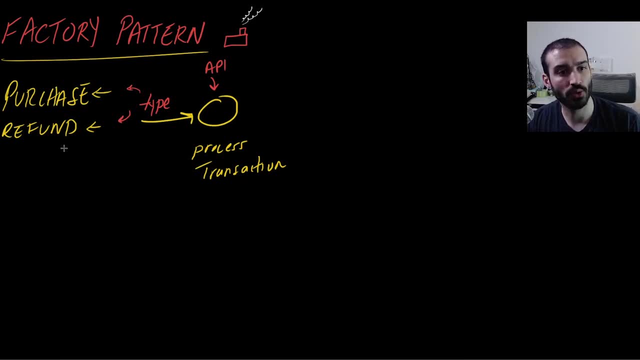 and refund. So let's say that we're building a transaction And let's say that we're building a refund. So let's say now that we need to write our handler of this API And the handler is just going to be the basic entry point for when this function is called. So what do we need to do here? 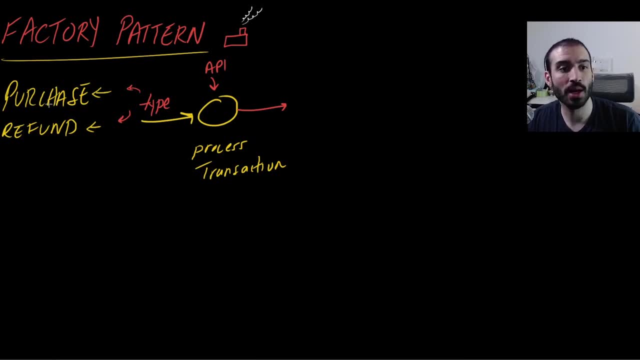 first in this handler. Well, our prerogative is to create the correct type of object that maps to these different enum values that are being passed into the API. So one of the first steps that we're going to do in this handler function is we're going to say if type is equal to purchase type. 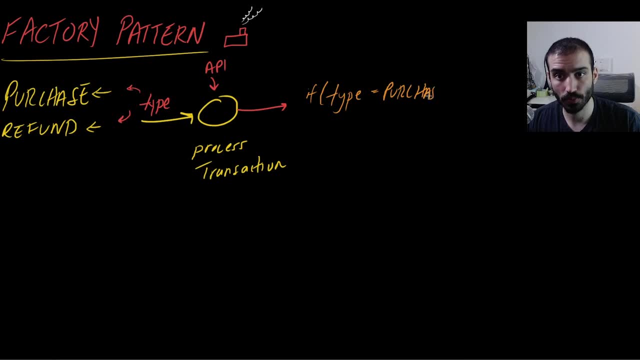 equals purchase. you know you're going to return a new purchase transaction or a purchase object, right, And then similarly you're going to have another line here or an else. if that also says if type is equal to a refund, then you return a new refund transaction. new refund transaction. 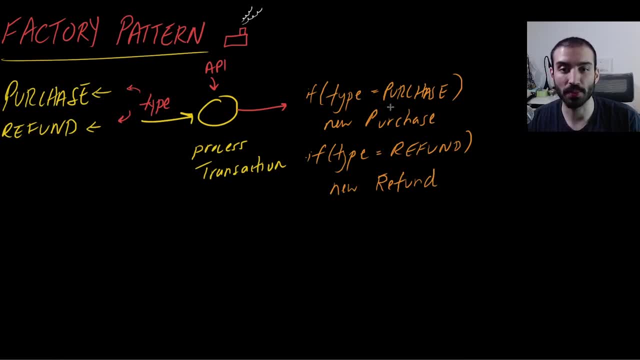 So what we're doing- this example- is that we're using these different if statements here so that we can correctly determine which object type to create. Now, there's nothing inherently wrong with the way that we're doing this. this is 100% correct. What we're doing here: 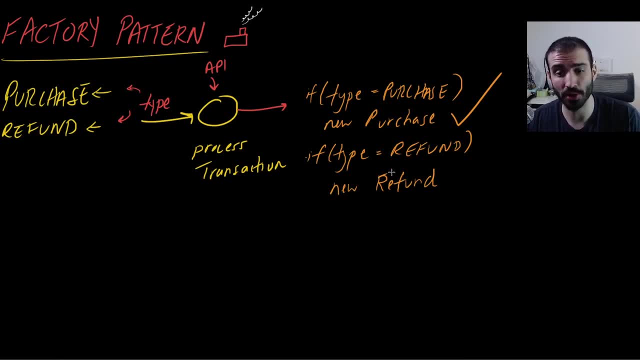 you know, with these if statements and this is actually how you implement the factory pattern, even it's in its more complex form, But this is the general idea of it And what you would typically do in the factory pattern implementation would be: you wouldn't have this. let me just mark. 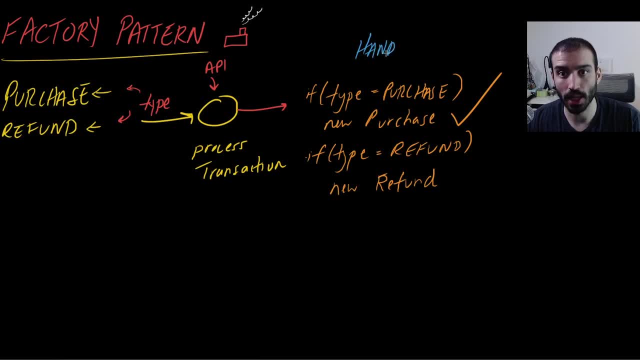 here that this is your. you know your, your handlers main entry point. you wouldn't have this code in your handlers main entry point. you would kind of take all this stuff out and put it into a class And then the handler function would call a method on this class that it can create the right. 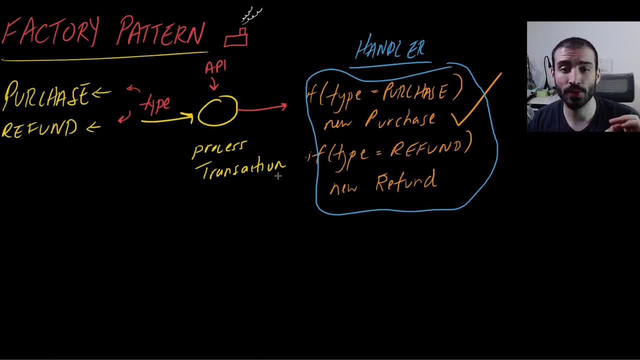 type. So this is the- you know, top level idea of the factory pattern. Its goal is to encapsulate object creation in another object. So that you know, in this example, in our handler function here, we don't need to worry about the mechanics of how to create our objects, we just need to know. 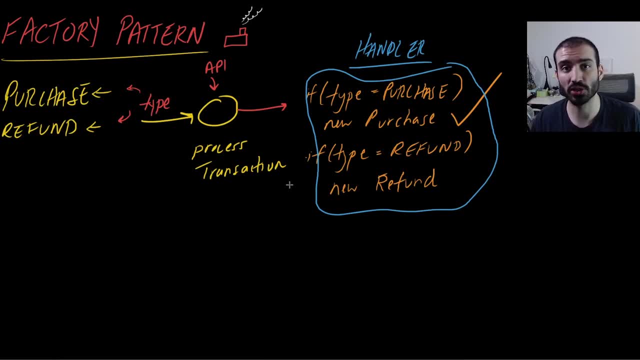 that, hey, if we need to create an object, all we do is we call this function in this method and it's going to give us back the right type based on the type that we pass in. And that's the general idea of the factory pattern. And if you think about this, like what? 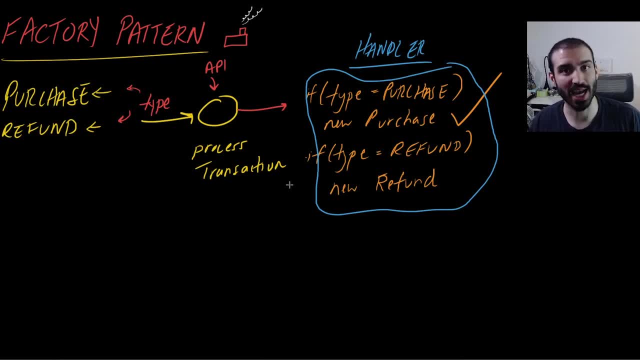 what I just described to you. I'm sure that you face this type of problem through your own coding methods. You know like this is a very, very common thing, where you're given some kind of type and you need to figure out what to do next with it and which object to create, So right off the bat. 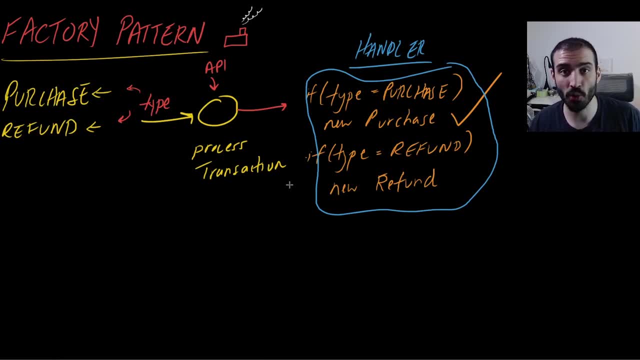 you can start seeing the value of this thing. you may not have known that this is a design pattern. you may have already been doing this in your code, But you know this is the, the building block of the factory pattern. Now, this isn't the complete factory pattern. This is what I call the simple. 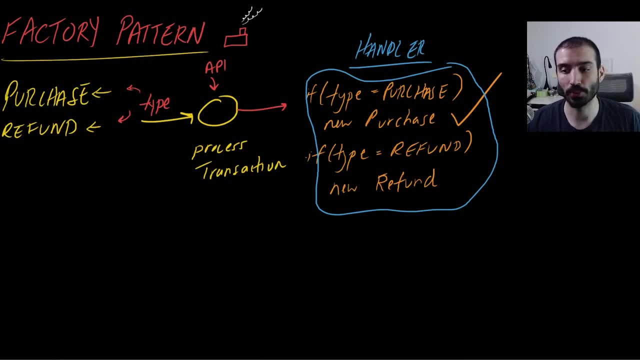 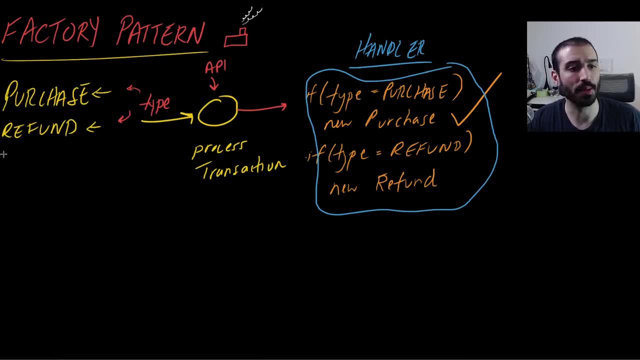 hypothetical examples. So let's think about some hypothetical examples Here. Let's say we introduce like a new type, maybe it's like a modification right mod, if, if occasion- and I apologize for my writing here in advance- it's really hard to use a tablet right on the computer. 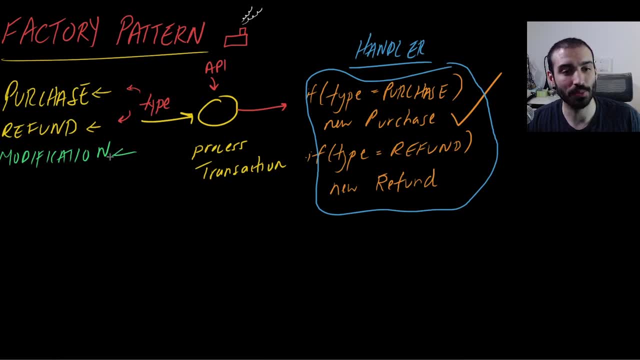 as it turns out. But anyways, say, we introduce, like this, new type here, And what do we have to do now in this handler function to make it work? Well, it's pretty obvious, right? we just need to add another if statement. if type is equal to, you know, modification, I'm not not going to write out. 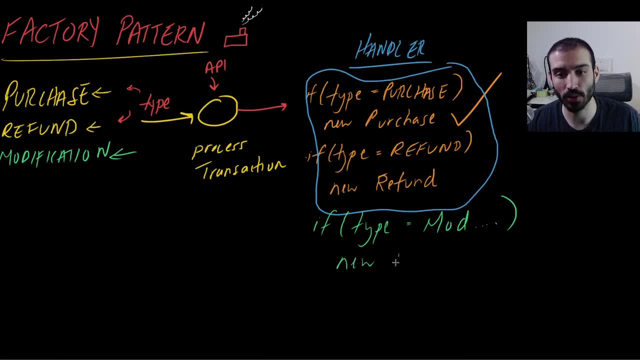 everything here. you know what I'm saying. then you're going to have to return a new modification, But this approach violates an important design principle. It's the O in the solid principles, And if you don't know what those are, go and check out my first video on design patterns. 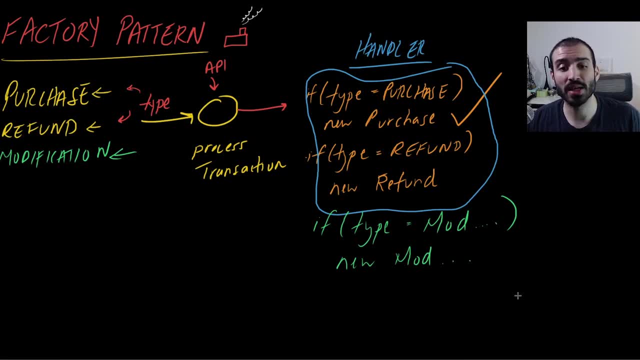 because I talked about them quite a bit. But what this violates is the open- close principle, And what the open- close principle says is that objects should be open for extension and closed for modification. Now, I've used the word modification here. that was not deliberate, actually, I just made this up on 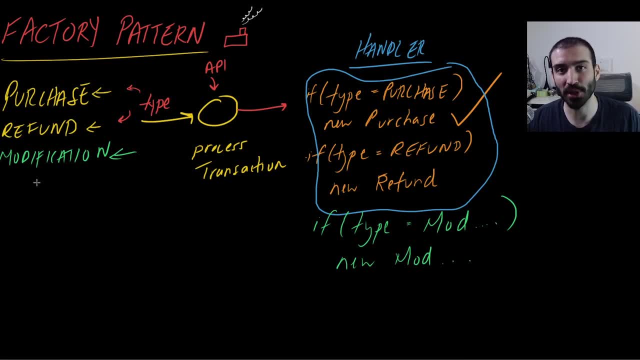 the spot and it happened to be the same word, But let me describe what that this, this open, close principle, means in the context of this example. Well, now, every time we want to create a new type of transaction, we need to go into this low level code. well, it's not very low level, but we need. 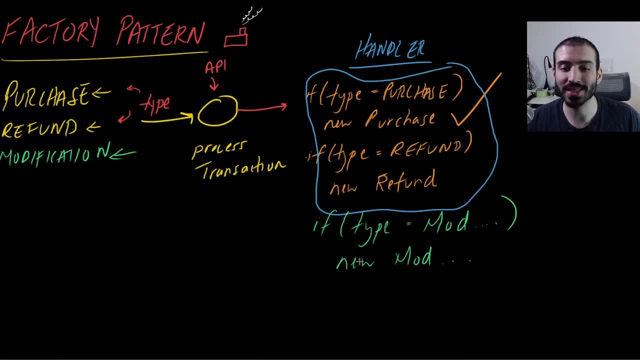 to go into this code and modify it. So this violates the open- close principle, And what this means is that objects should be open for extension and closed for modification. Now, I've used the word open- close principle because we need to, you know, go inside and modify it So we're not closed. 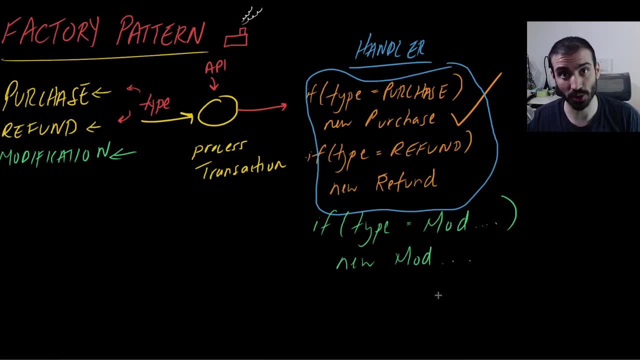 for modification. we are, in this case, open for modification, which is a bad thing from the open, close design principle perspective. Now, the way that you can get around this problem and still adhere to the O in the solid principles, well, there's two approaches actually. 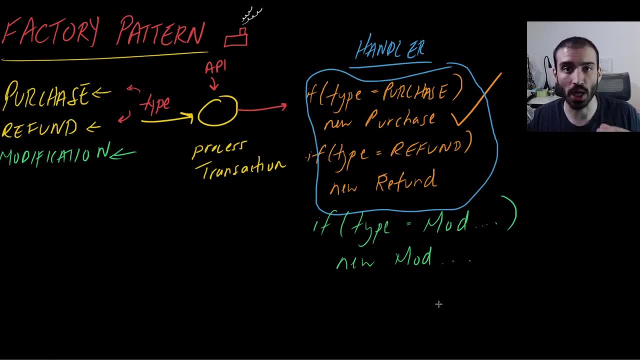 the first one is using inheritance and the second one is using composition, And in this video we're going to talk about the inheritance form of the factory pattern And the next one I may talk about the composition form of the factory pattern, which is a little bit. 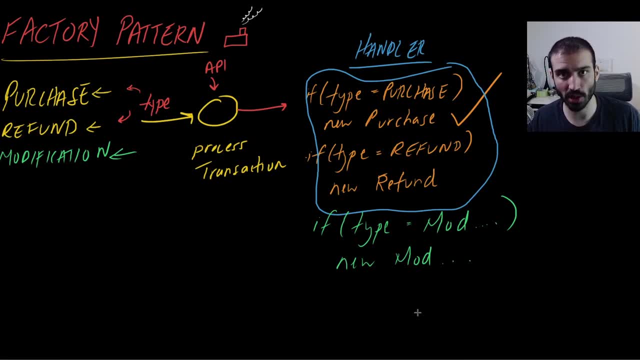 more complicated, But I just want to make sure that you get the idea here And you can start applying this stuff to your daily work. So, just to recap everything that we talked about here: the factory patterns for object creation delegation- and it's useful so that we 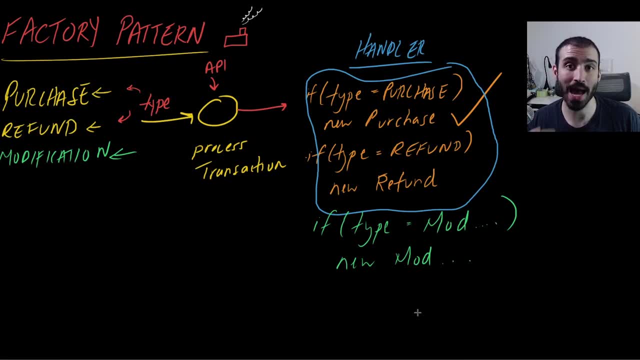 can offload the responsibility of how, the mechanics of how to create an object, to another class whose sole responsibility is to know how to create objects. That's the factory pattern that we're going to be using in pretty much one or two sentences. So let's scroll down a little bit And I want to talk to you for a few moments about. 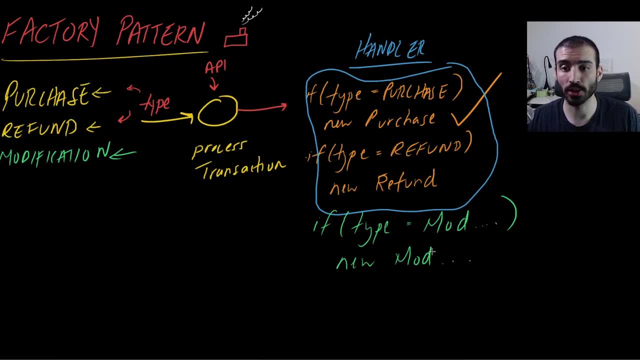 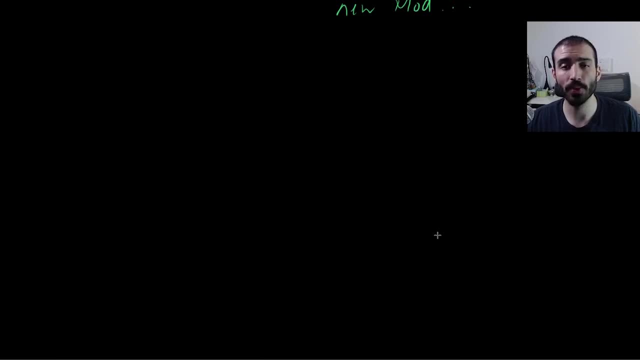 the example that's used in this book because that's the one that we're going to be using to go through the code in my ID in a few moments And the example is a little bit different. they are using like a pizza shop example And we're just going to kind of run with that and 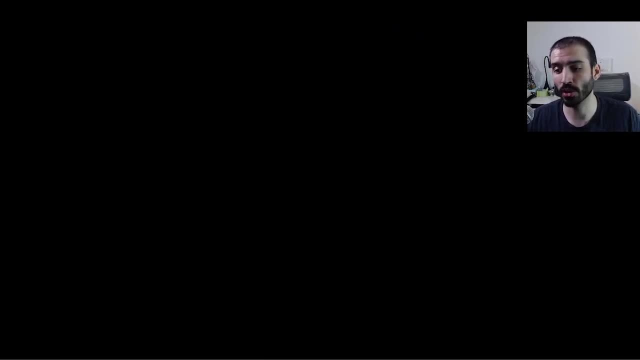 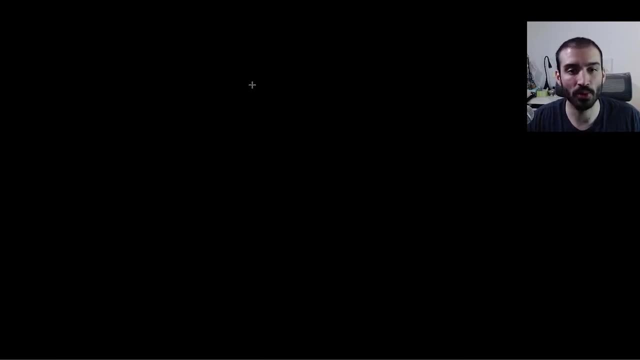 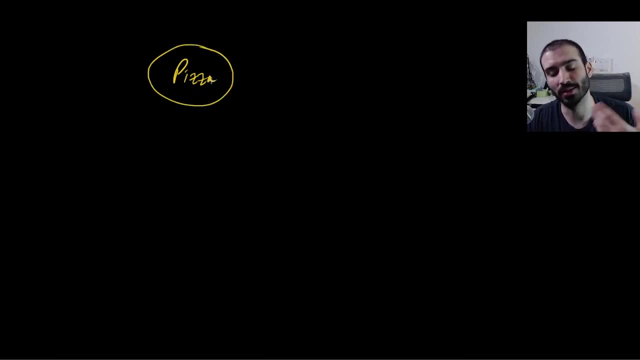 creating instances of, And this isn't going to be like a complete class diagram here. this is just going to be some quick notes that I throw together, So keep that in mind if you're reading this. Now. a pizza has different methods that need to be performed on it. So the first step: 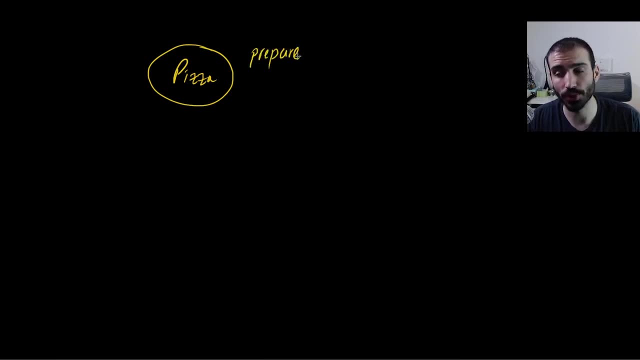 is to prepare the pizza- this could be like rolling out the dough. The second one is to bake the pizza, So actually throw that in the oven. And the third is to cut the pizza. And the last one is to box the pizza right. So these are the four main operations that we perform on a pizza in. 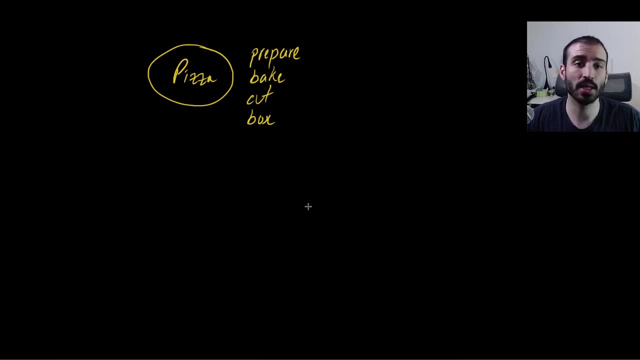 order to make one right, And in this example the pizza is going to be an abstract class. abstract class And we're working in Java here. So if you don't know abstract classes they're kind of like a formal class, But basically it's kind of like a classical class where the problem is. 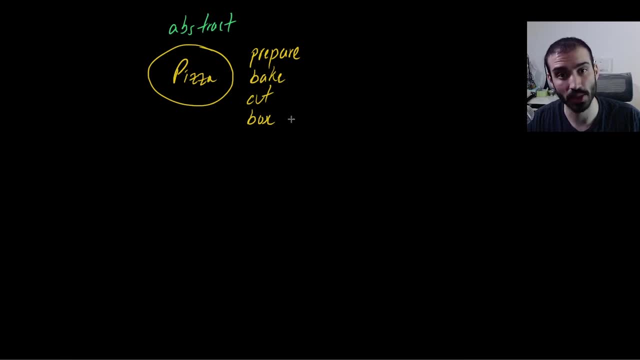 you know, you could have a pizza that's like a very, very basic pizza, but it's not necessarily going to be an abstract class, because it's probably going to be a very, very complex pizza. So then the third step is to create different variations of pizza, And in order to do that, 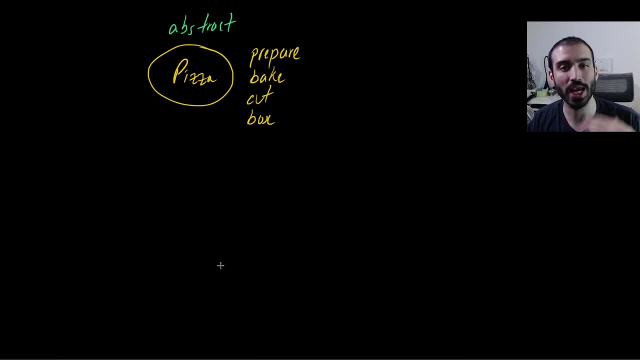 I'm going to be providing you a basic example of what an abstract class is going to look like. So we're going to be looking at a pizza, or a large size pizza, or a large sized pizza as we would call a fondant pizza, or a large sized pizza, And what I want to show you here is 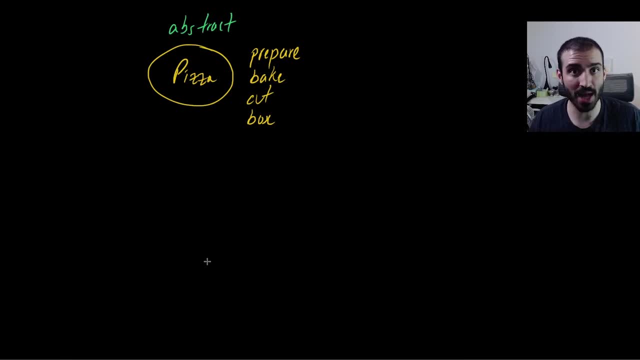 pizza is like a very deep dish pizza and maybe like an italian chain where you typically get very thin crust and very crispy style pizza, and those are different types of pizzas. they may have the same properties in terms of, you know, the same toppings, but they are different types and maybe 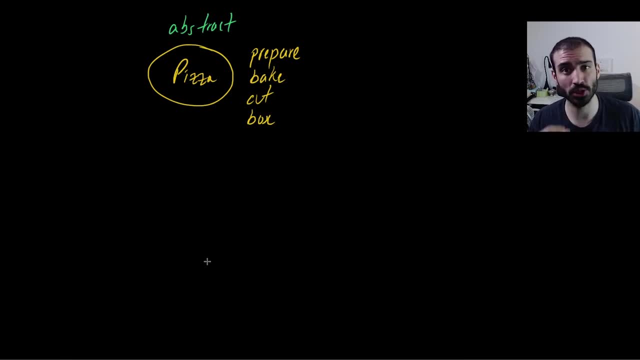 there's different ways to actually create those pizzas, in terms of the dough, the cooking time, all that kind of stuff. so in the, in the book, they go through how to kind of set this, this structure, up, and so what they suggest is to create two different subclasses of the pizza. so we have 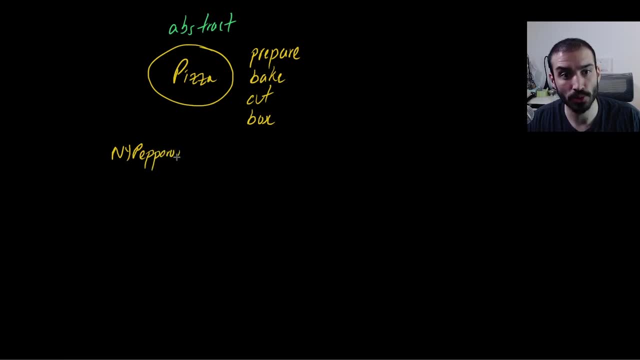 a new york pepperoni pizza. new york pepperoni pizza and a new york cheese pizza. right, and you can obviously add many, many more examples of this, but let's just keep it to two in this example, just to keep things simple. now we have a relationship like this: so new york pepperoni. 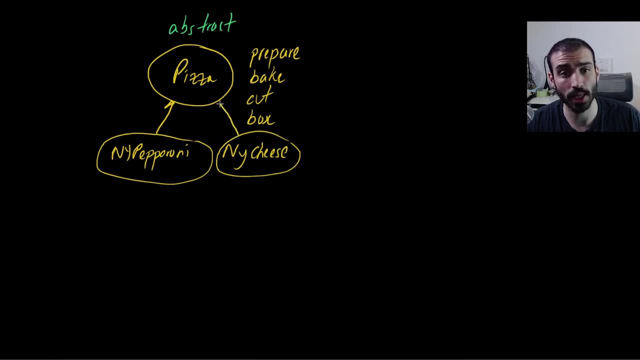 implements the pizza inner or the pizza abstract class. i should say so the new york cheese and new york pepperoni. they need to define how to actually prepare, bake, cut and box right, because they could be different depending on which type of subclass is actually implementing the pizza abstract class. so that's the main idea here and you can imagine what this 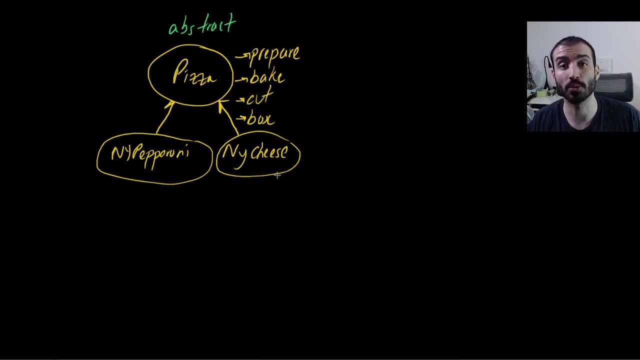 looks like if you add multiple different chains or multiple different franchises. here you can add, like, an italian one out over here, and now it can implement the abstract class. you can add a chicago one out over here, and this kind of goes back to what i was telling you about before with the open- close principle. 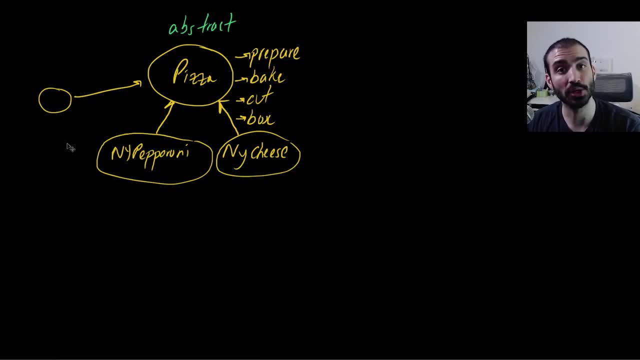 so we're not using any kind of modification here to create new types. we're just extending the pizza by creating new instance types through this inheritance relationship. so so far we haven't really got to the point where we actually use the factory method or the factory pattern. we're 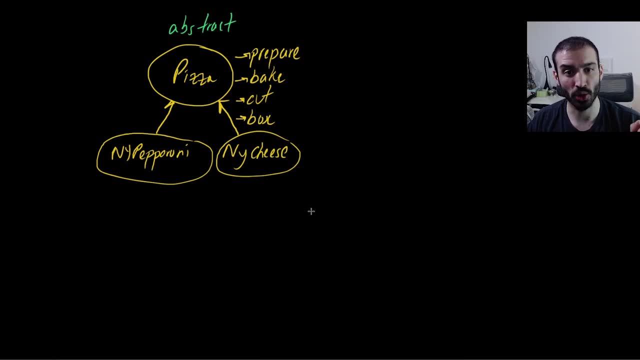 just kind of setting up the classes so that we can work with them in a coherent way later on. so just to to kind of emphasize here: so new york pepperoni, new york cheese, these are both concrete classes, concrete classes. so you're going to be instantiating these two now in parallel. 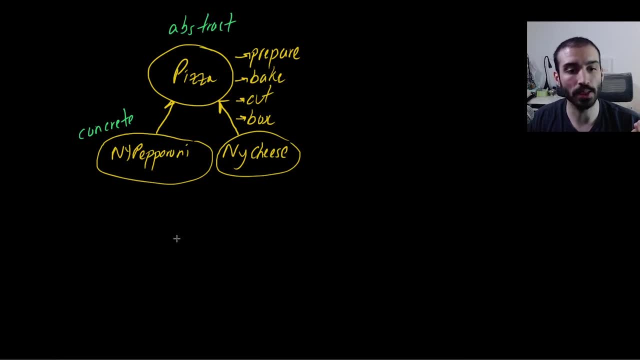 what you have going on is this concept of a pizza store, pizza pizza store- right, and this entity is going to be, in essence, your factory, right, and you can call this a factory, like you can call this a pizza factory or you know whatever you want, like if it makes sense to use. 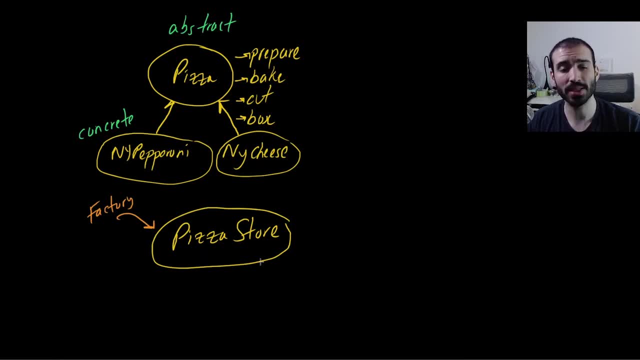 the name factory, like i don't think it actually does in this case. but basically, whatever object is going to be responsible for object creation or containing the logic for creating these objects, that's your factory object. in this case it happens to be a pizza store, and with our pizza store we're 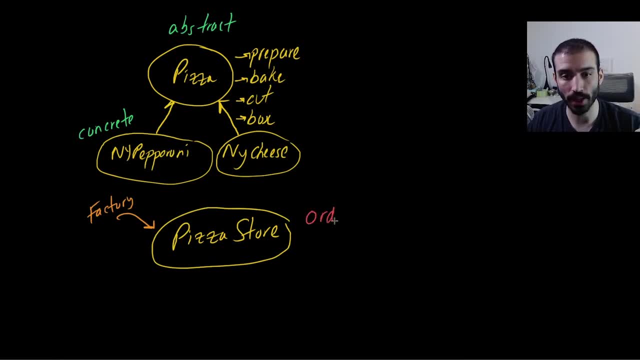 going to have two different types of methods. we're going to have the order pizza method, order pizza method and this is going to take the type and if it's, you know, cheese, pepperoni, whatever. it's not going to know like a new york style and it's not going to know a new york. 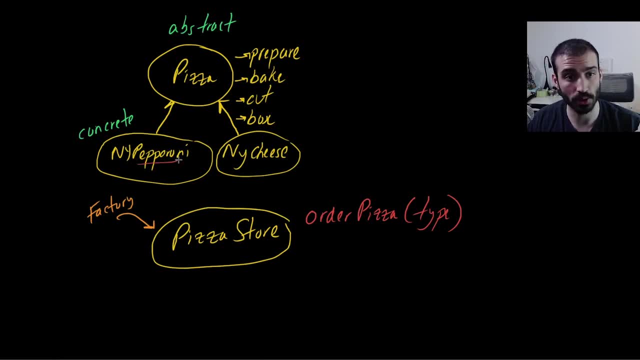 pepperoni, but it's just going to know like cheese or pepperoni. so let me just underline those, just so that it's clear. that's what's being passed in here, not the new york style pizza. so that's going to be the first method, and then the second one is going to be creates pizza, and i'll explain to you. 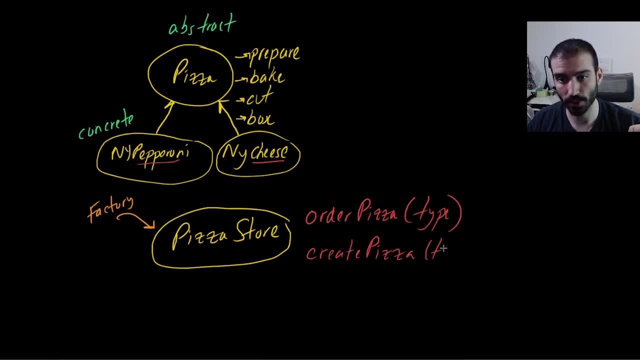 why we have these two different things in a moment. here just one. let me get this hashed out: type: there we go and of course, there's a siren right now. all right, so that finally passed, thank goodness. now going into why we have these two different methods, so let's talk about that for a moment. 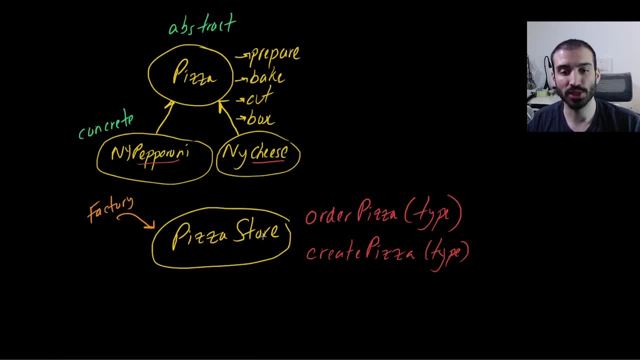 so in our pizza store or in our, in our example, in general, we always have the same sequence of operations that take place. we always want to prepare the pizza first, then we want to bake it, then we want to cut it, then we want to box it right, and that is consistent across any type of pizza. it doesn't matter if it's a new york style. 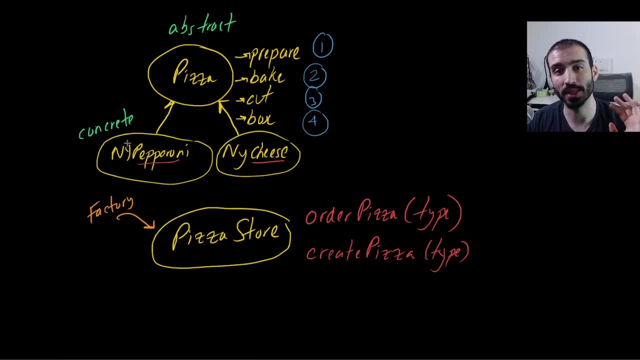 pizza, pepperoni style pizza, an italian pizza, chicago pizza. that pattern stays the same and it never changes. so what the order pizza method is going to be responsible for is it's going to be calling a method that which is the create pizza method and passing along the type it's going to. 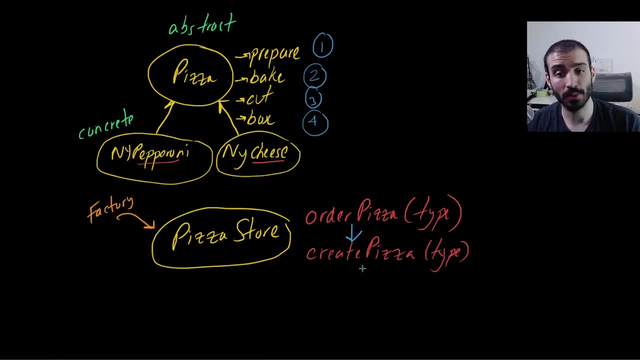 get an instance of your pizza object and then perform an order and then it's going to be going to perform these steps: one, two, three and four. so it's going to call the prepare method, it's going to call the bake method, it's going to call the cut method and it's going to call 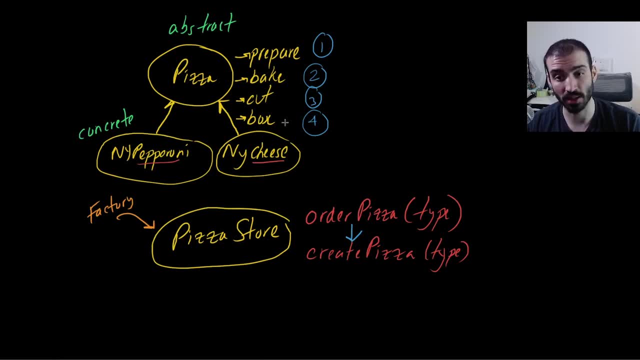 the box method before it finally returns that object back. so the create pizza method. this is actually the the important bit here, because this is essentially the the factory method that you're going to be using to store the logic of you know if pepperoni, then create a pepperoni pizza. if 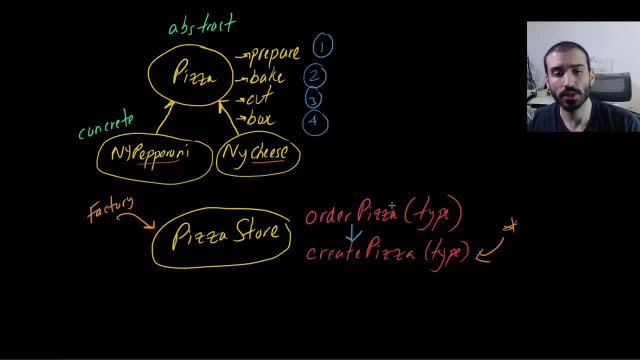 cheese pizza, then create a cheese pizza, and then create a cheese pizza, and then create a cheese pizza, so on and so forth. so what's going to happen here is that the order pizza method in the- well, this is an abstract class. perhaps i should have mentioned this before. we're going to have a 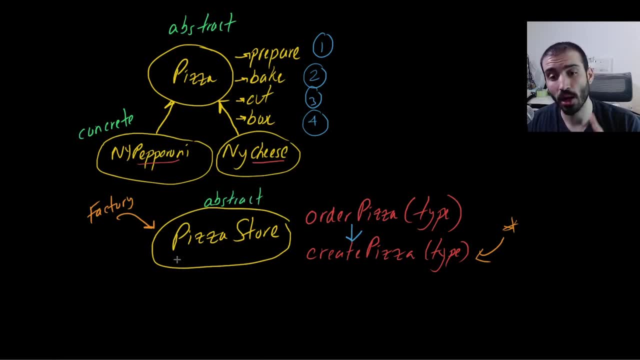 subclass here. that gives us more granularity on the type of pizza. i'll get to that in a moment. but in our pizza store method, because we're following the same operations generally for most types of pizzas, we can implement the order pizza method to perform these four things in. 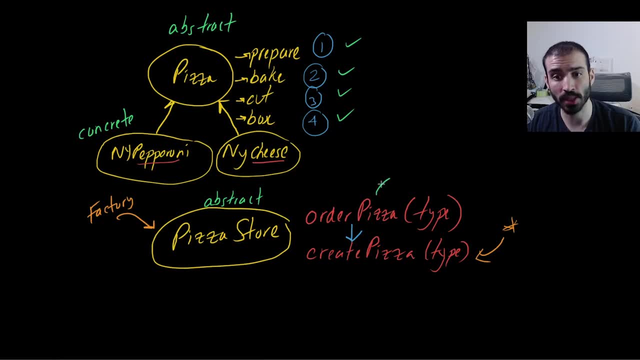 sequence. so these are both going to be abstract methods and we're going to be following the methods, but the key is that this one is going to be implemented in the pizza store- abstract class implemented and this one is not going to be implemented. so it's going to be up to the 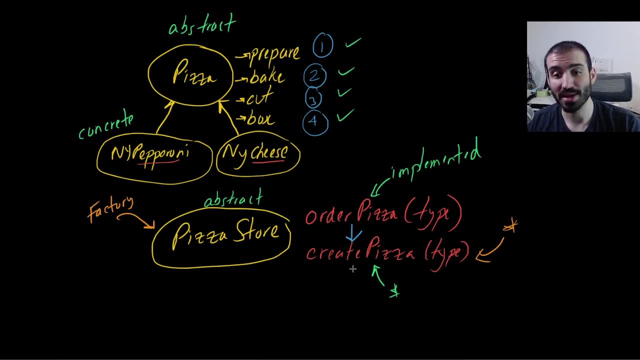 subclass to define the create pizza method. now, that's important, and i'm going to show you why in the next step. so that was the setup. now there's one key element that i left out and you're probably wondering, like: how do we connect, you know, the concept of new york cheese style pizzas with this? 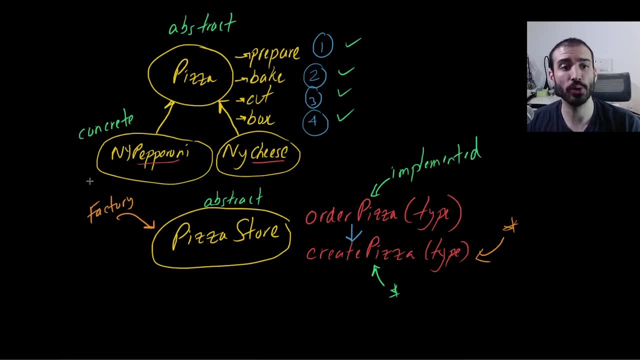 concept of the pizza store, like: how do we tell it to create new york style pizzas, or italian style pizzas, or chicago style pizzas or whatever, right? well, the way that we do that is we have different subclasses that implement the pizza store abstract class. so, in order to create new york style pizzas, 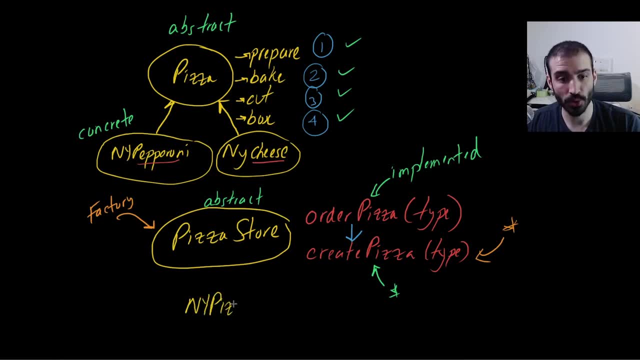 we have a new york pizza store, new york pizza store right, and this is a child class of the pizza store, so i believe the arrow goes in the middle of the pizza store and then we have the in this direction, and so what happens here in this relationship is that the new york style pizza. 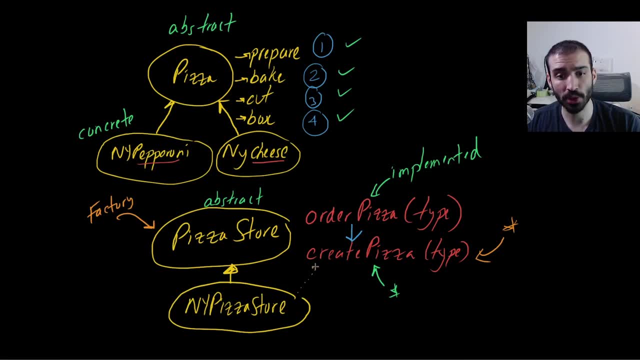 store. as you may recall, it needs to implement the create pizza method and it needs to handle the different types that new york style pizza supports. so in this case, it supports pepperoni and it supports cheese. so what it'll actually do is, in its kind of create pizza method, that it's going. 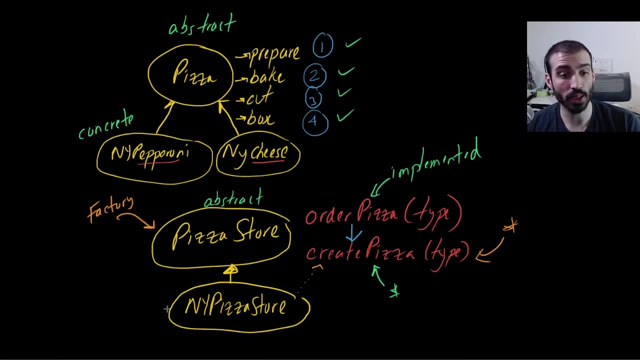 to define it's going to have. you know, if it's pepperoni, then you create the pizza store and a new york pepperoni pizza, and if it is cheese, then you create a new york cheese pizza. and you can quickly see where i'm going with this. and let me just um kind of backpedal on those so i can. 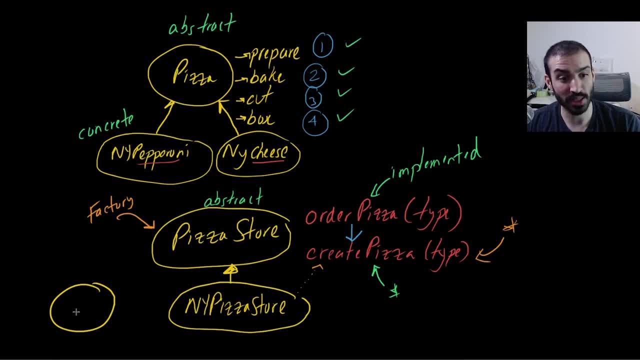 clean up the diagram a little bit here. you can create other ones as well, like the italian pizza store, italian pizza store, right and. and use the same kind of pattern. now and uh, the italian pizza store follows the same pattern. it implements the pizza store and it defines its own. 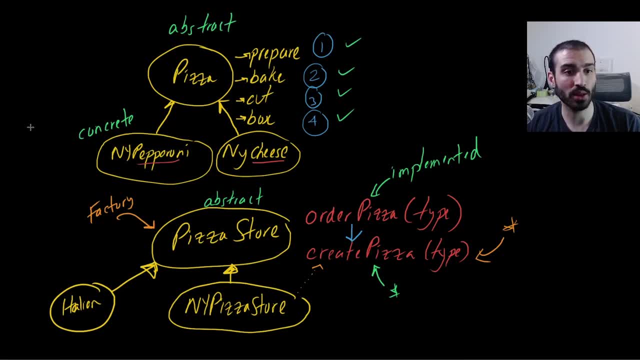 method of creating pizza, uh method, and then that can create the italian pizzas, so italian pepperoni, and then your italian pizza store is going to be instantiating instances of the italian pepperoni pizza. so this is the essence of the factory pattern. so just to recap on everything we talked. 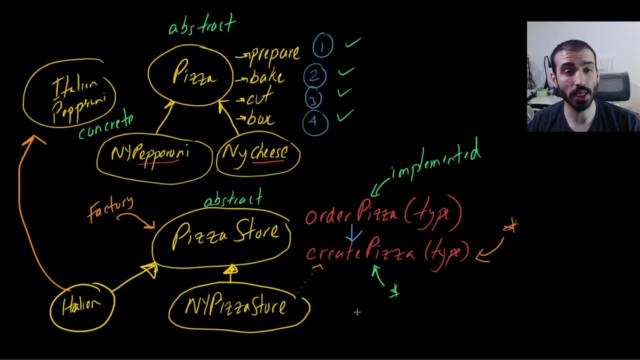 about here before we get into the actual code in the ide. so we're working in a pizza shop example. we have a pizza store and we have a pizza store and we have a pizza store and we have a pizza store abstract class, and that has four different methods and that includes prepare, bake, cut in box. 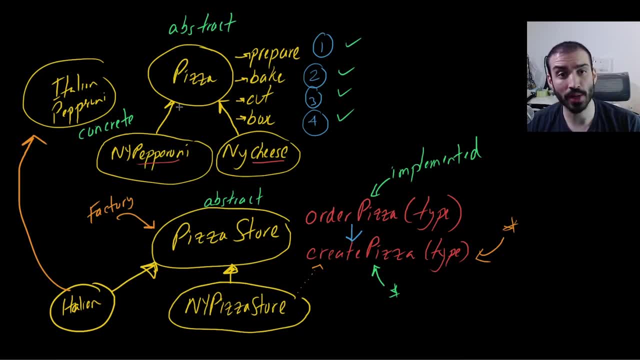 we have different types of pizzas that implement this abstract or extend this abstract class. i should say new york style pepperoni, new york style cheese and any other type that is specific to a certain style or franchise. and separately from that, we have a pizza store which acts as a factory. 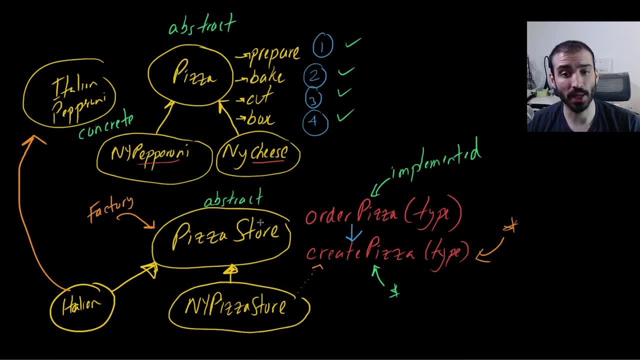 in this example, and we have, and this is abstract, by the way- and the methods are. there's two methods: order pizza, which has a default implementation, which prepares, bakes, cuts and boxes the pizza in that sequence. it also calls the create pizza method of the underlying subclass, which knows. 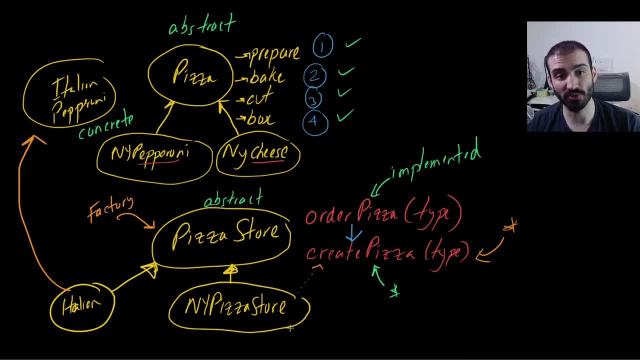 internally how to create the different variations of pizza, whether that's a new york cheese or a new york pepperoni, and of course that depends on the type of factory. in this case, because you know, the italian pizza store in the new york pizza store are the subclasses of the pizza store and the 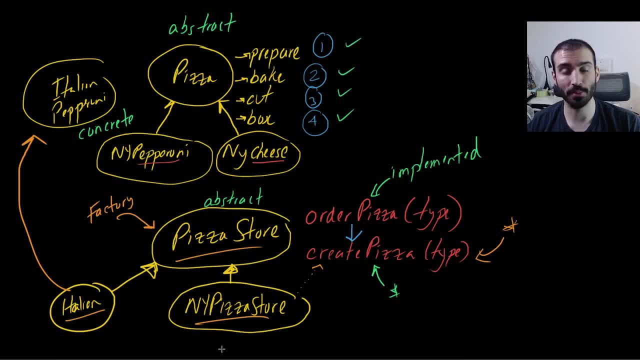 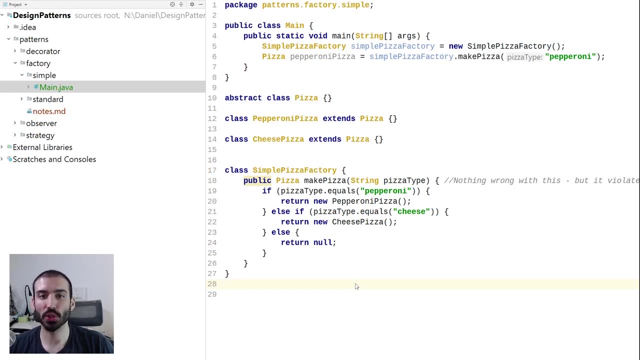 factory class, which is the pizza store in this example. so i hope this was clear, and if it wasn't, don't worry about it, because we're going to go into the code now and i'm going to show you exactly how this works, using just a basic setup for a java application. so here we go. all right, guys. so here. 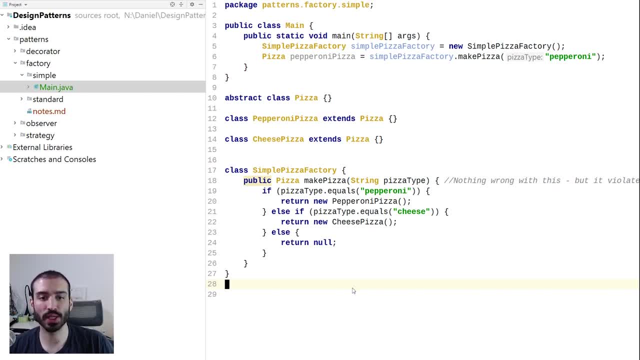 we are in my ide. so i have two little examples that i just wanted to show you. the first form is the super basic example that is similar to what i was showing you in the purchase transaction at the beginning of the video. just to show the most basic form of the factory pattern. i call it. 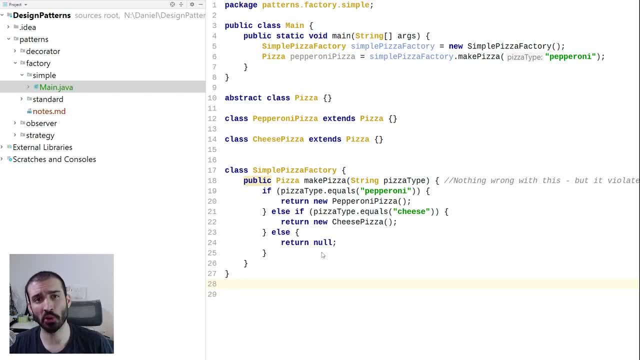 the simple factory pattern. and, by the way, i'm going to be making all this code available. so if you want to, you know, play with this- i'm going to put the link on github in the description section below so you can check it out there. so let me just show you this example really quick before we get into 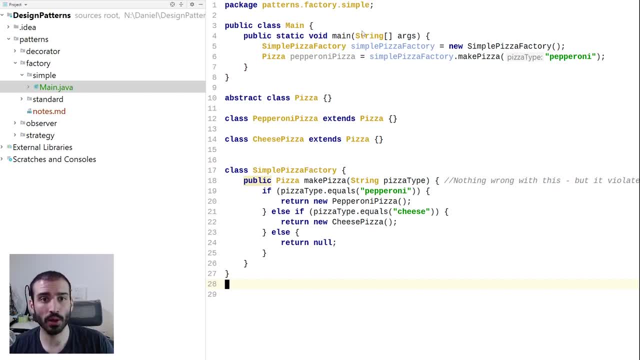 the other example, which is a little bit more sophisticated. so ignore this stuff up here which is our runner. so bear with me. here i have a couple different classes that are defined here, but i want each one of them to you. so we have our abstract pizza class, we have our pepperoni pizza, which 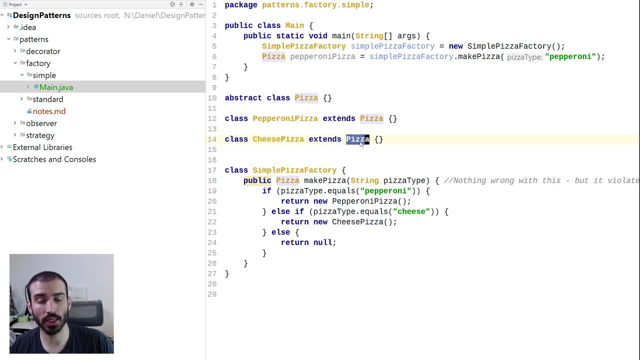 extends pizza. we have our cheese pizza, which extends pizza as well, and then we have our, our factory method here, our factory class, and this has one method. uh, it takes the pizza type, which can be, in this case, pepperoni cheese. maybe you want to be veggie, anything else, and as i'm kind of calling, 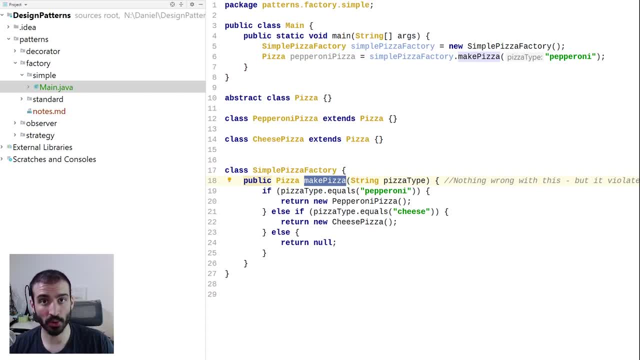 out here. there's nothing wrong with this, but it violates the open, close principle, and we saw an application of that in the the blackboard method. so we're going to be using that method and we're going to be using the blackboard example that i was just showing you. uh, so, if you see what this 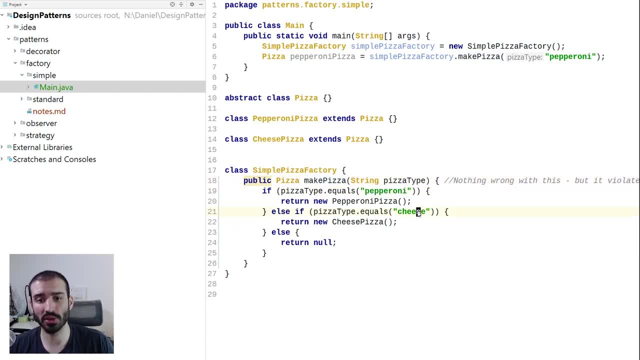 looks like it's very, very simple, right? you just look at the different types here that are being passed in and return the new instance as it matches the type that's passed in. and if we look at the runner really quick, what are we essentially doing? well, we're creating an instance of our pizza. 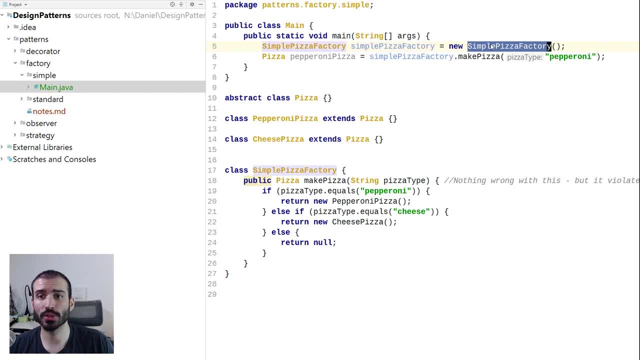 factory which, in the example before, was the pizza store. and then we're just, you know, creating an instance, and then we're calling the make pizza method, and then we're, we're getting a method, we're getting an instance of the pepperoni pizza because we passed in pepperoni. 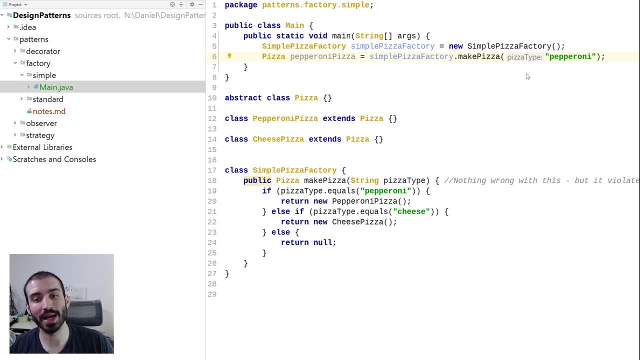 so that is the most simple implementation of the factory pattern. let's move on now to the example that we were demonstrating, the second half with um, the pizza store and everything that's involved there. so let me minimize that and we're going to go into standard here and let's walk through all. 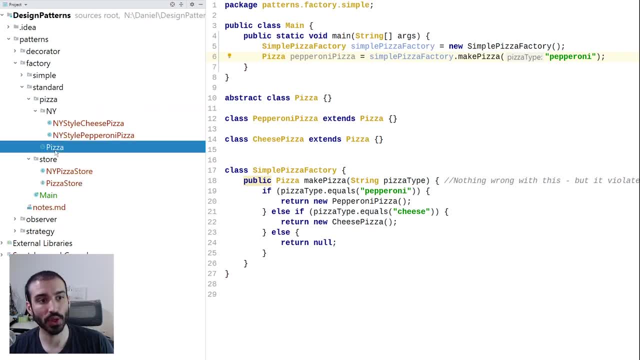 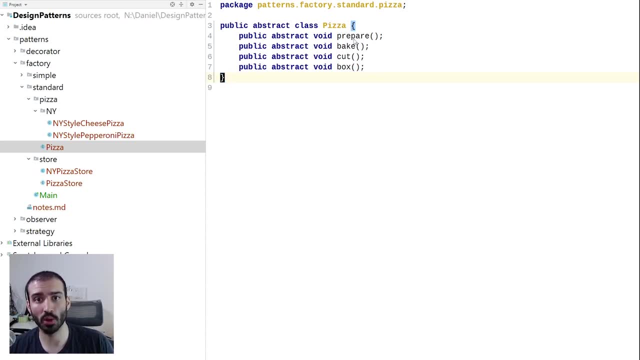 the classes. so let me expand all these guys out so that you can see. so, first of all, we have our pizza class. this was our top level entity and it has these public abstract methods. so prepare, bake, cut and box. and if you're not familiar with java, if you're using abstract here and you're defining it in this way, you're. 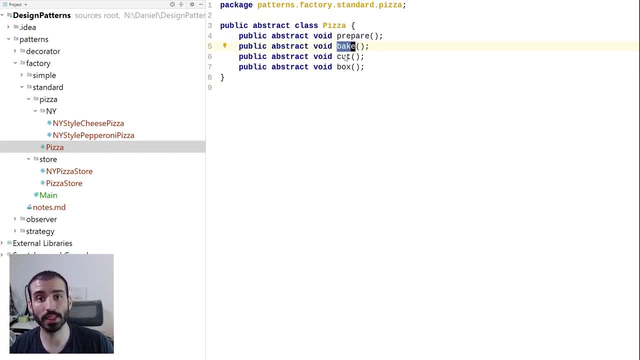 basically saying that the subclasses much must define this, these methods, in order for the program to compile. so then we also have these two types of pizzas. in this example we just have two types for new york and just kind of organize this in a pretty coherent class structure. so if 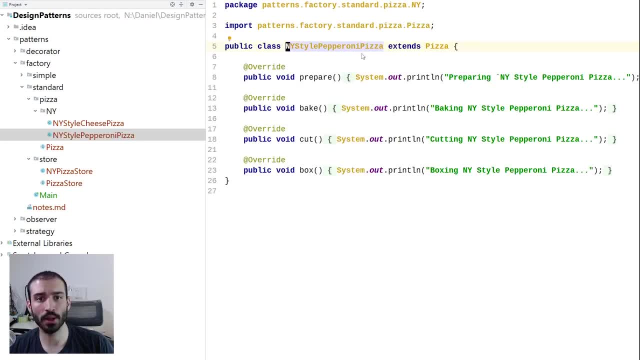 we take a look at the pepperoni style pizza now we can see that the new york style pepperoni extends pizza. it calls the prepare method or defines the prepare method. i should say- and you know we're not doing anything sophisticated in here, but you can imagine where preparing a new york style pizza is. 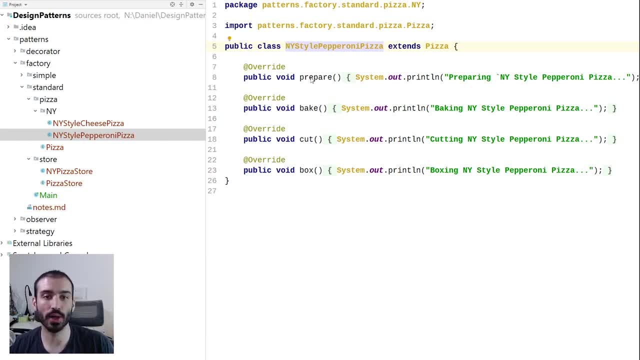 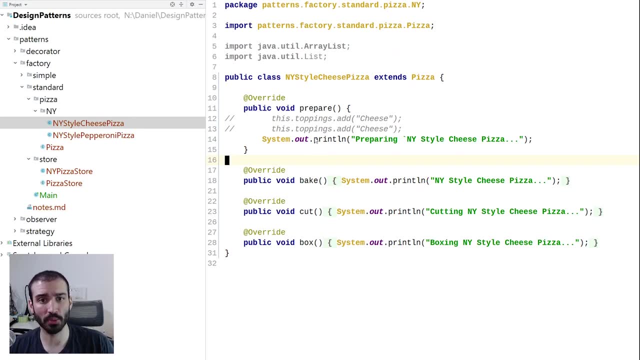 very different than preparing an italian style pizza, so on and so forth, and that can be different for each of these different methods here. and i'm kind of hinting at that in the next example where i introduced this concept for the cheese pizza of topping. so say, you had like a toppings array, that 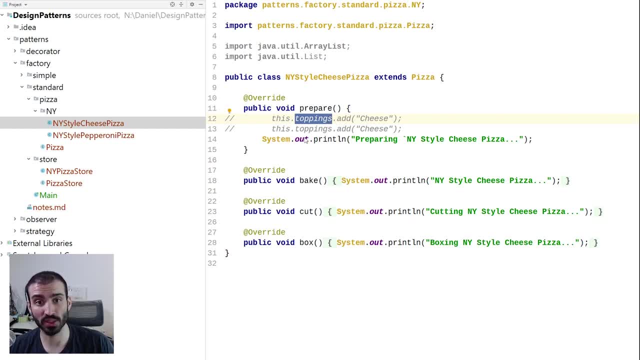 defines the, the ingredients or the toppings for this pizza. so in the new york cheese pizza, you may add extra cheese, because that's what's specific about new york style pizzas. or if it's a chicago pizza, it may be thick crust, so you may have to define a property giving information about the crust and 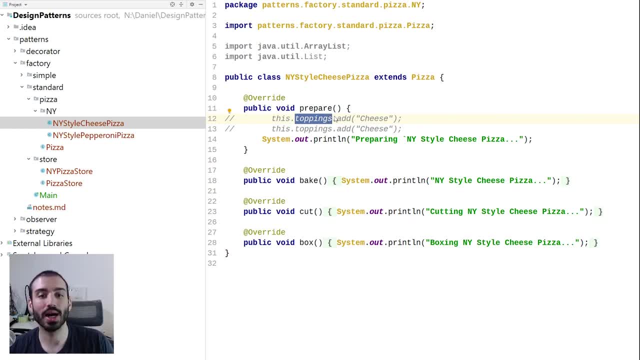 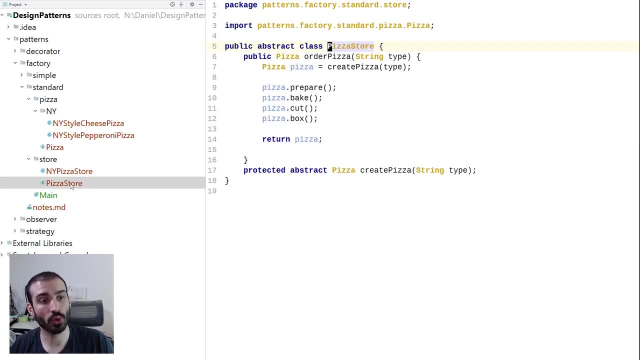 and say that for the chicago style it's a thicker crust. so that's the general idea here. but they're basically following the same kind of pattern if we look at the pizza store, which was, if you recall, the kind of most important part of this equation. so it is a abstract class. it's got the order pizza method and the create. 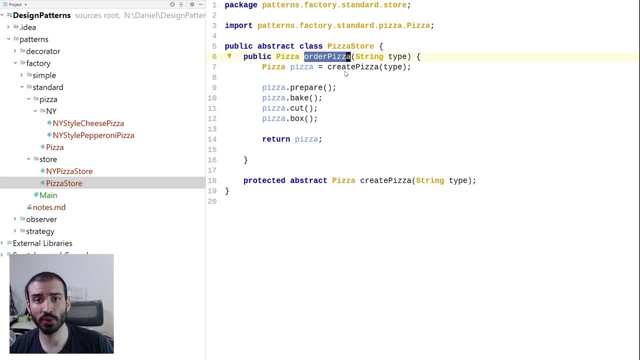 pizza method and it's got a default implementation of order pizza and the first thing it's doing is calling the create pizza method. and the reason why this is important is because the pizza store is going to be subclassed by the new york style pizzas, chicago style pizzas, whatever, but this 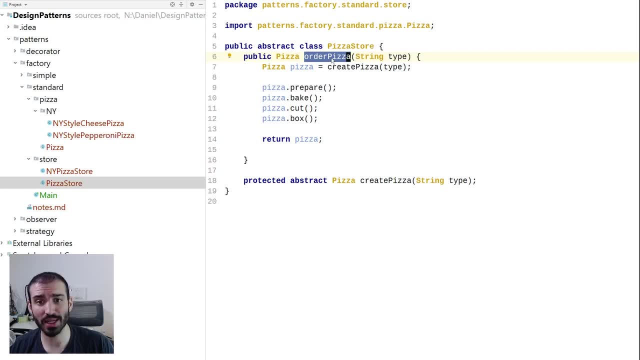 method does not need to know the order. pizza method does not need to know how to create the pizza. it just knows the order of operation, and that's the one thing i'm going to talk about in a. So it doesn't know how to create the instance. 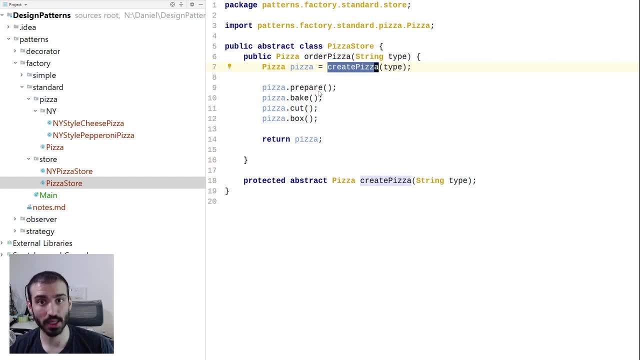 it just knows how to operate on the instance. So that's where the real key here. So this thing here, this create pizza method, which is not given a default implementation, is the key to this puzzle. So, as we see, here, you're just creating the instance type. 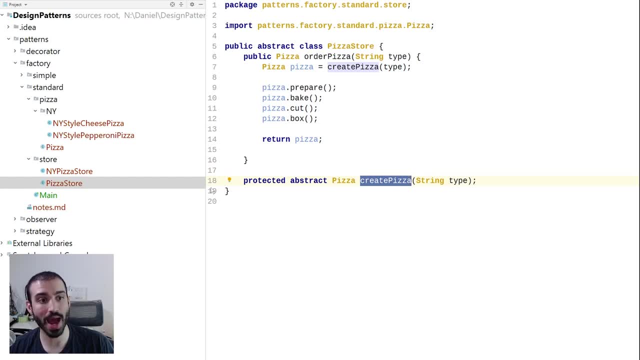 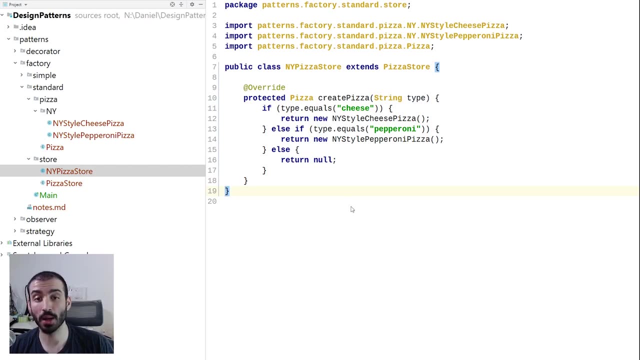 and you're calling your operations on it and returning that back. Now, if we look at the New York pizza store, this is where that kind of a pseudo code if statement from the beginning of the video kind of comes into play, And this doesn't really change all that much.